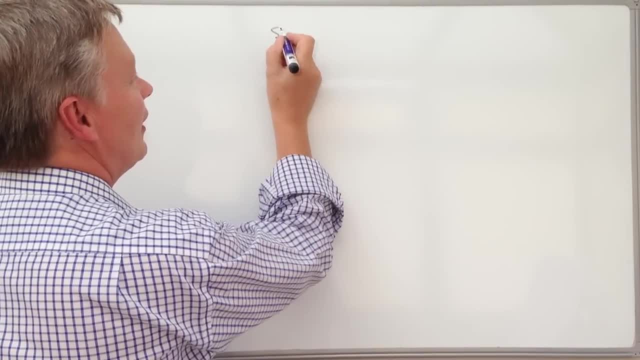 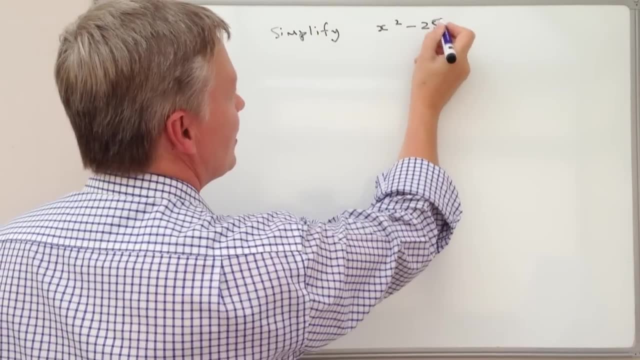 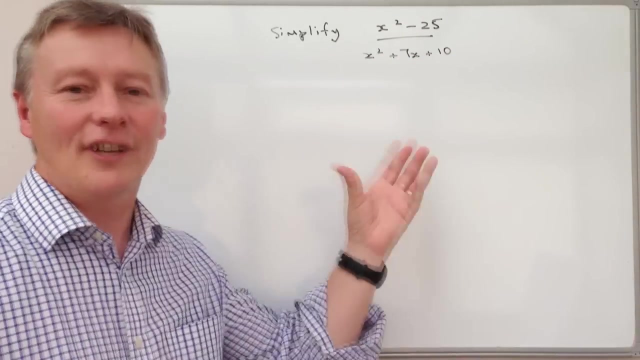 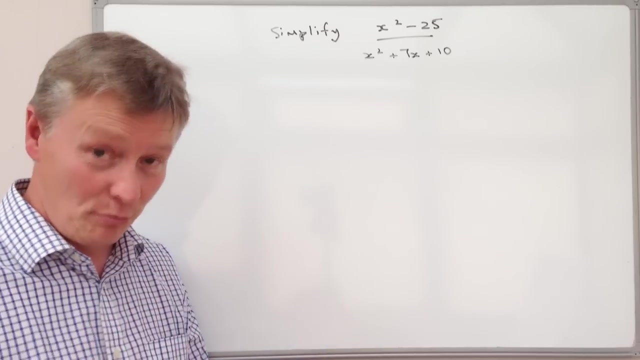 The way that they'll be written. it will say something like simplify, and it's going to be x squared minus 25 and that's going to be divided by x squared plus 7x plus 10.. And when you first look at these it can look a little bit intimidating, but actually, if you break it down into its component parts, it's not too bad. 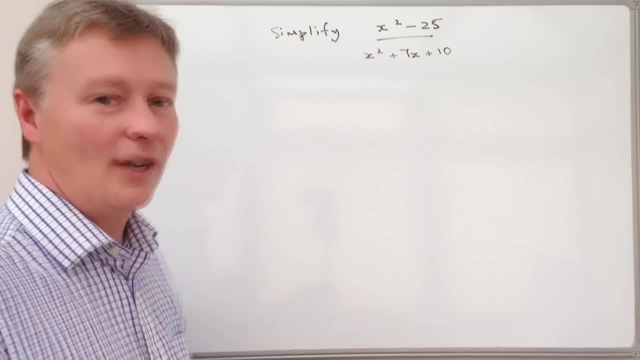 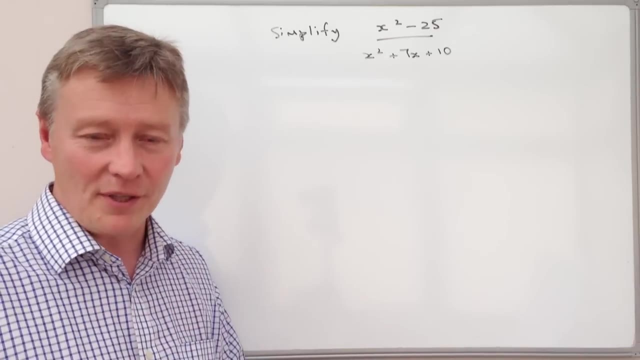 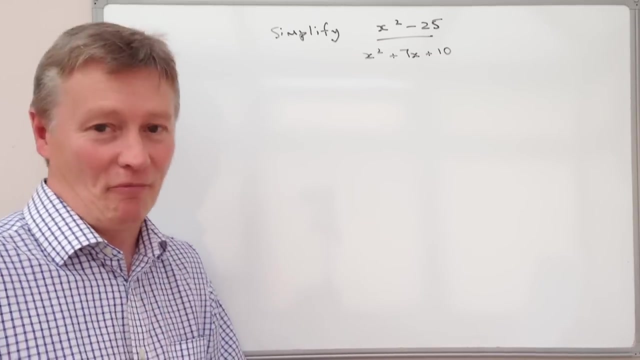 The main thing with these is you need to remember that with in keeping with every fraction, whatever you do to the top of the fraction, you've got to do to the bottom. So if you divide the top by something, you've got to divide the bottom by the same something. 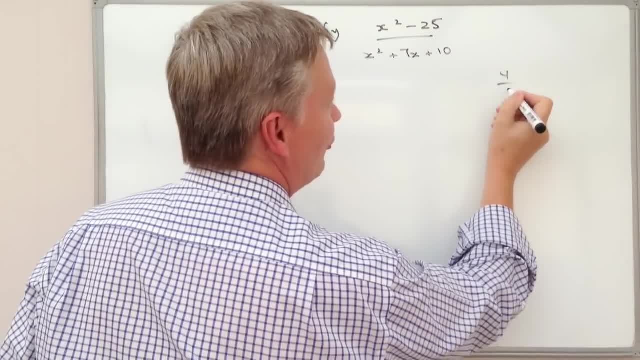 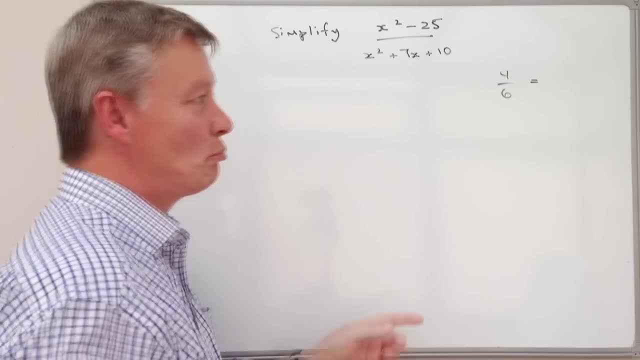 So, just as a very brief example, let's say you've got 4 over 6.. Well, 4 over 6 can be simplified by dividing the top and bottom by 2.. So if I divide 4 by 2, I get 2.. If I divide the bottom by 2, I get 3.. 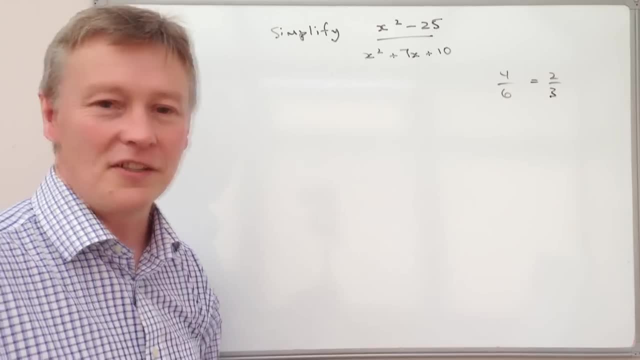 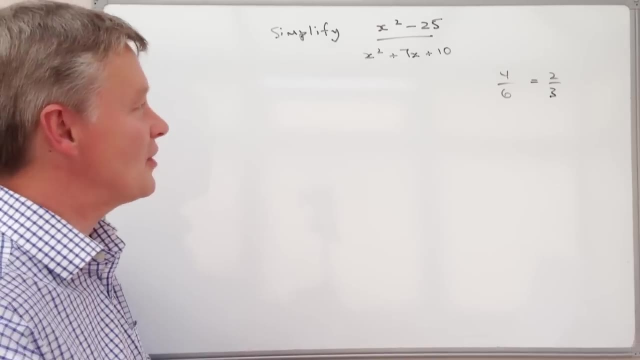 And it's a little bit easier to deal with 2 thirds than it is to deal with 4 sixths. Okay, so what we're going to do is use the same sort of principle with this, But the first thing we're going to do is we look at the top bit, which is the numerator. 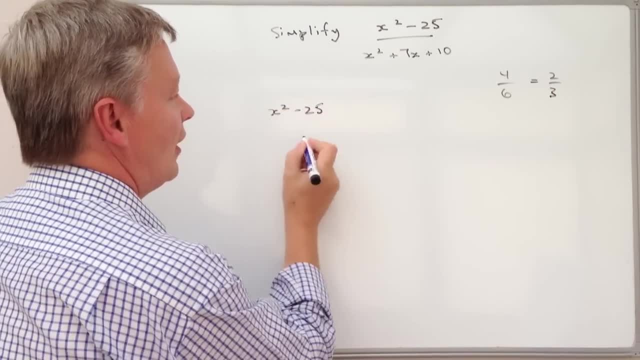 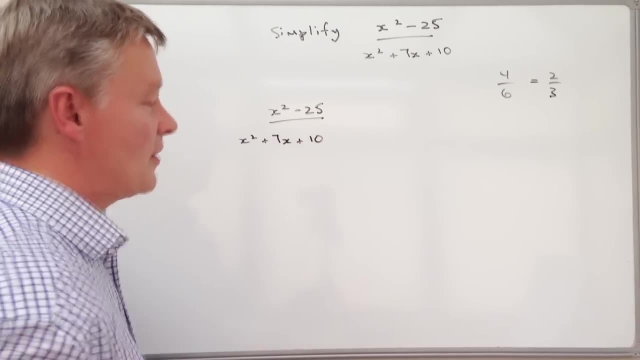 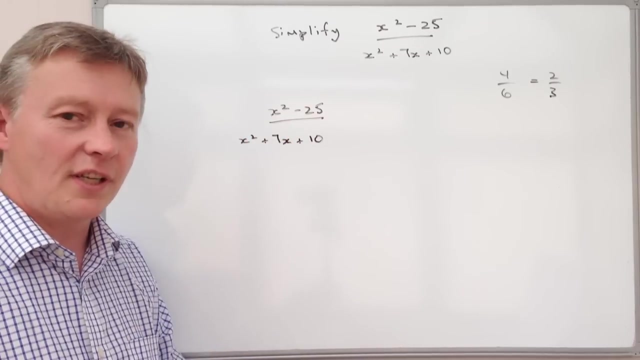 And we've got x squared minus 25.. Okay, and if I just write out the whole thing again, I've got x squared plus 7x plus 10 on the bottom. Well, the main thing to remember, or to to to look at, is at the top. this particular one is the difference of 2 squares. 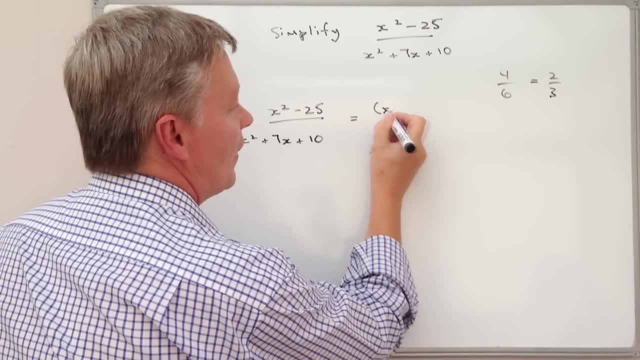 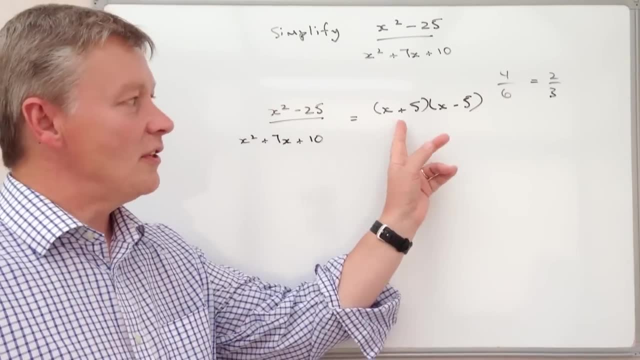 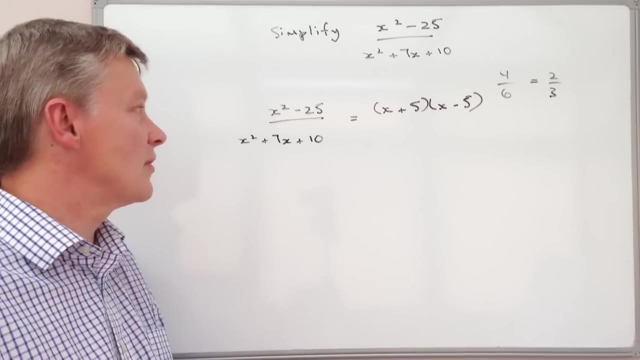 So if I factorise that, it's going to be x plus 5 and x minus 5.. Okay now, if that's not quite clear to you, then maybe you need to have a look at one of the other videos. And there is another video on difference of 2 squares. 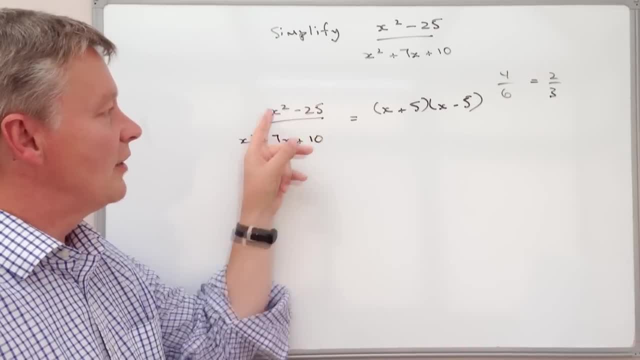 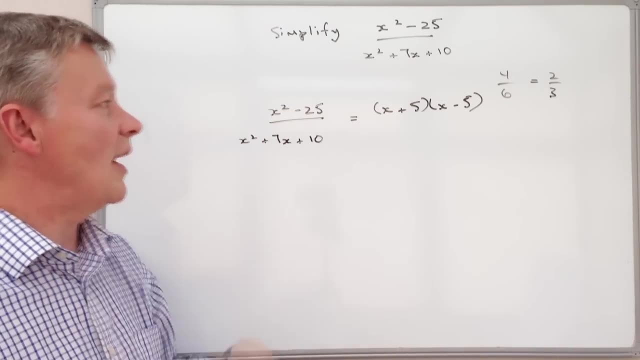 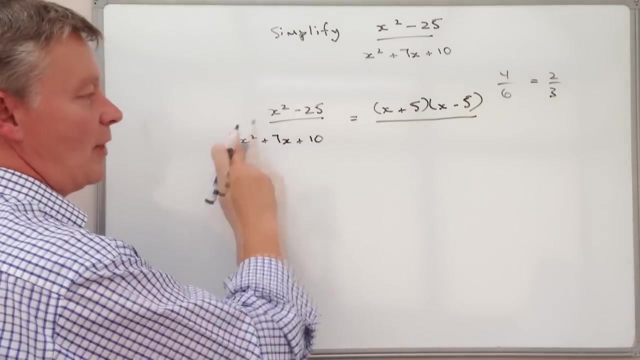 But basically what we're doing now is taking the factors of that and if you multiply that back out, you'll see that it actually does work out to x squared minus 25.. I'm going to do the very similar thing with the expression on the bottom.